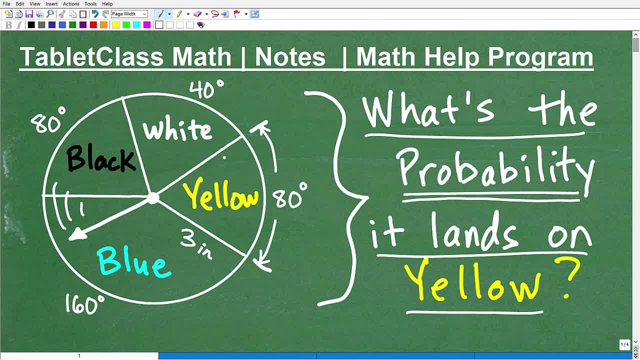 little sectors. right, This is an arc of a circle, But these are like little slices of a pie. So here we have 80. And then our blue is obviously bigger. So this is 160 degrees. And then over here we have a black which is also 80. And then this little white sector which, let's say, is 40. So it's not a perfect figure, But you know, hopefully this problem is making sense. So we're going to solve this problem in just one second, But first I'm going to quickly introduce myself. My name is John. I'm the founder of 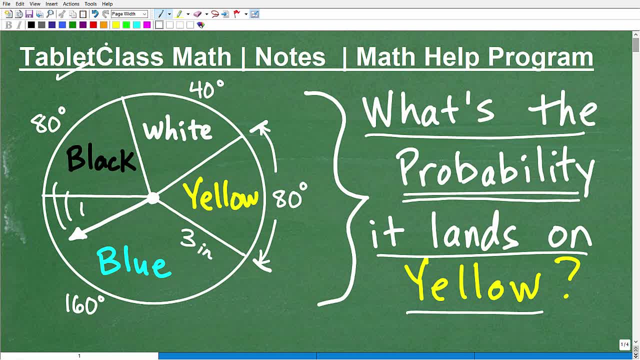 Tabaclass Math. I'm also a middle and high school math teacher And over several years, I've constructed what I like to believe is one of the best online math help programs there is. Of course, I'll let you be the judge of that, But whether you need to take a full course or you need assistance in the course that you're in, my math help programs consist of very, very comprehensive lessons- okay, much more than what I do on YouTube- And I literally show you how to solve thousands of problems. Okay, so, 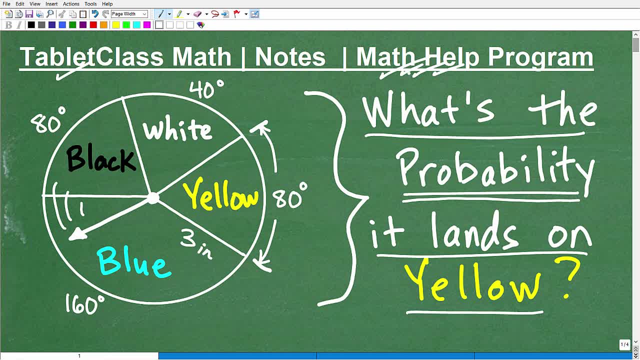 again, this has taken me years to construct and build Because, you know, being a math teacher, I know what students really need to successfully learn math, especially more advanced mathematics. Now one of the things that you need to be doing- irrespective of whether you want to check out my program or not- is, if you want to do well in math, you absolutely need to take great math notes. So, over decades of learning or teaching math, one thing that I've noticed- and it's kind of like my golden rule- is those students who take great math notes. 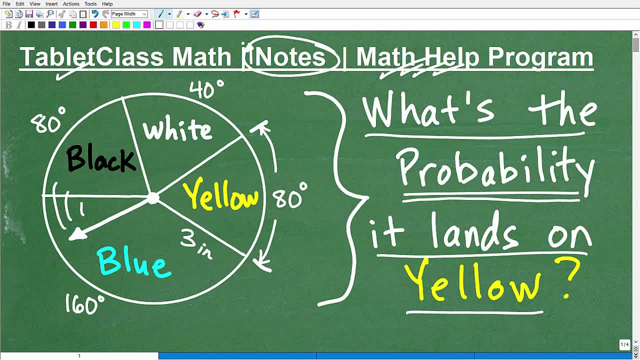 almost always have great math grades, And the reverse is true. Those students who don't take any math notes, or sloppy math notes or unorganized math notes, or maybe your dog ate your homework and your math notes. whatever the case might be, you kind of get the idea here right. So if your notes are anything less than outstanding, you need to work on them, And it is a skill. it takes time. I definitely wasn't a strong note taker. I was terrible even in high school, because I really didn't, you know. 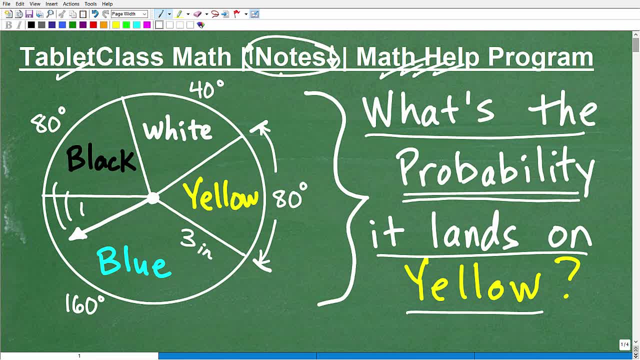 pay attention. you know, wasn't interested Because I thought to myself: I don't need math, I'm just gonna, I'm going in. I went right into the Marine Corps. I wasn't going to college after high school so I said, what do I need this for? But of course, later on, you know, I wanted to go to school and study mathematics. you know I found out pretty quickly. you've got to take great math notes. But in the meantime, if you don't have great math notes right now, you can get a set of my math notes. okay, very detailed, comprehensive. those would include 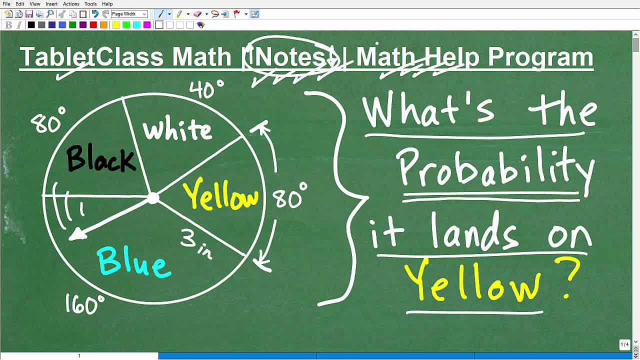 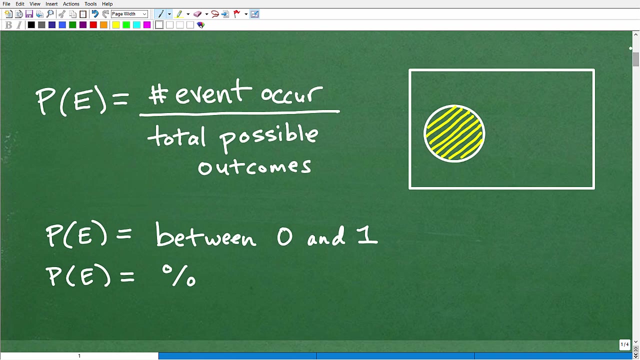 pre-algebra, algebra one, geometry, algebra two and trigonometry. you can find a link to those in the description of this video as well. Okay, so let's get into this problem. Obviously, we're dealing with this topic of probability And this is just a simple probability problem. Okay, probability is a big topic, And so I'm going to kind of quickly review basic, simple probability concepts And with this particular problem, 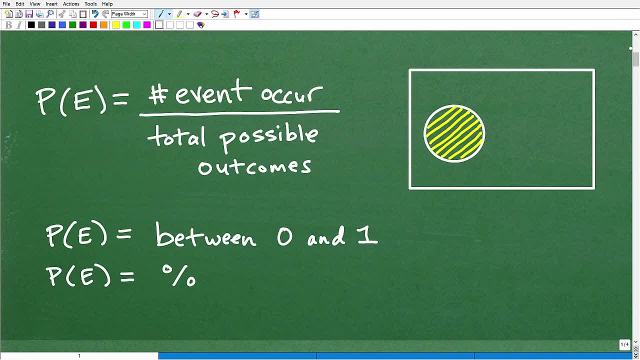 we're dealing with kind of kind of a figure, okay, so I'm going to talk about this little little diagram, this little figure, here in a second as well, because I want you to be familiar with how to handle these type of basic probability prompts. Now, probability, okay, as a general definition, we kind of write it this way: this little P of E does all this means is that the probability of an event occurring, okay. So what does that mean? Well, let's just imagine this thing. let's say this was a- oh, I don't know. let's say a wall. 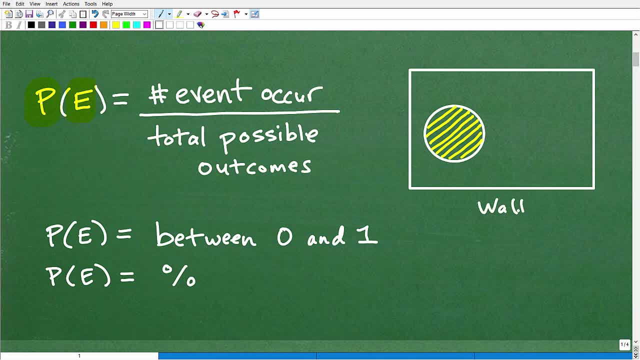 for lack of a better term. let's say, in some you know, bedroom of a house or this is just a wall, And you had this big old, like yellow circle on the wall. okay, like so. And let's say you're, you know, moving out, And okay, and you're like: hey, you have your, your darts. okay, you know what a dart is? right, you throw those things and they kind of stick into the wall, into a dartboard, right, Normally it would be like a dartboard. But let's say, you just want to throw a couple darts at this wall for whatever reason. okay, 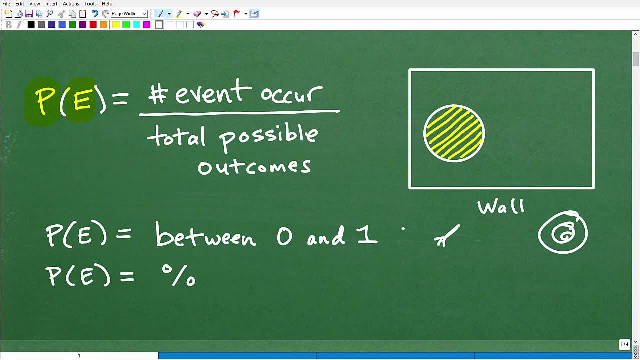 And you're standing back And you want to determine what is the probability that you, when you throw this dart, it will land in the yellow circle, okay, So the way we determine, okay, probability is the number of ways that particular event can happen. okay, So now with a dart, it's a little bit different here, because you're like, well, I don't know, this is like area right, But in general, probability is the number of way, number, the number of ways that particular event can happen. 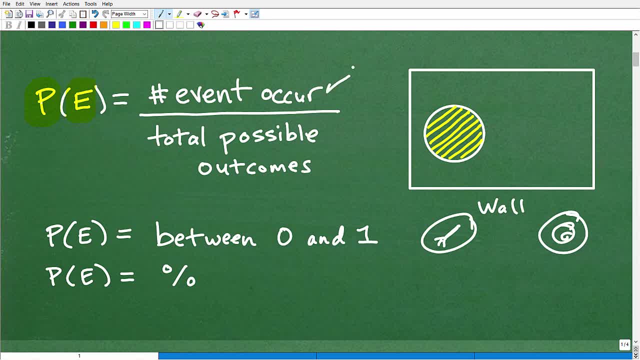 different ways an event can occur. okay, just in general kind of conceptual manner over the total possible outcomes of events. So here this is going to be a fraction. okay, it's gonna be some sort of fraction, And a probability is always going to be between zero and one. because we're talking about a fraction here, right? So where the denominator is one, all right. so our probability we like to express in terms of percent, So the probability of something happening like this. 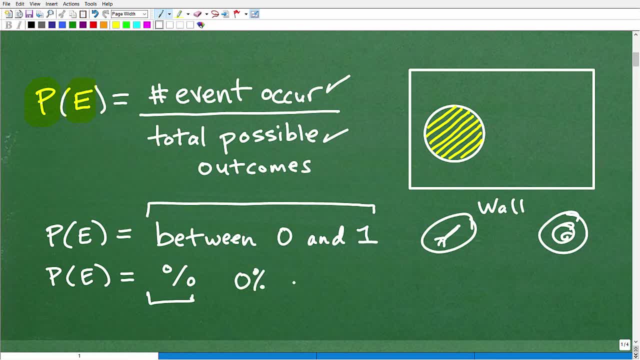 situation will be between 0% and 100%. Okay, so I want to explain this all with this particular problem Again, just trying to do a quick review of probability concepts now. So the definition of simple probability is: the probability of an event occurring is the number of ways that event can occur over the total possible outcome of events. But in this particular problem we're dealing with something kind of graphically going on here. 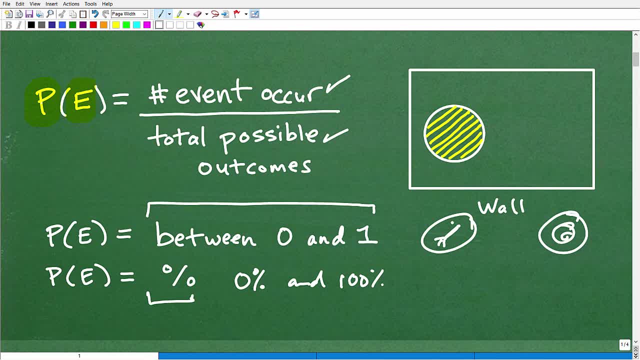 right, like a figure. So let me get back to our my little dart problem. So when you have a problem like this, okay, the total possible outcomes is what, if I throw this dart and it's going to land on this wall, it can land here, here, here, here, here. it could go, you know, in my little yellow circle, here, here, here, here. So the total possible outcome is this entire rectangle. okay, But we'd like to 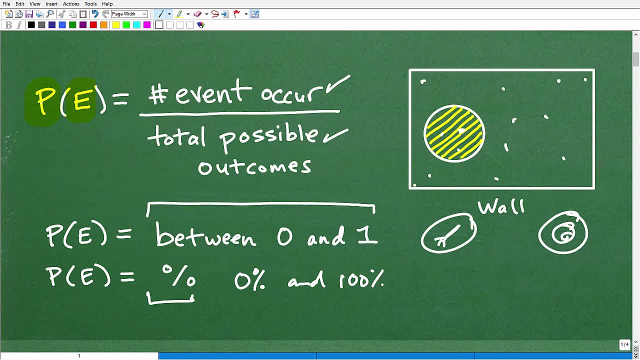 use area. okay to represent the total possible outcome when we're looking at something graphically like this. So the entire area of the rectangle in this particular kind of little basic problem would be the entire area of the rectangle, Okay. Now, if we want to determine what's the probability that's going to land in this yellow circle, we want to find the area of the circle. Okay. so this is going to obviously be less right. the area of the circle is less than the entire area of the rectangle. 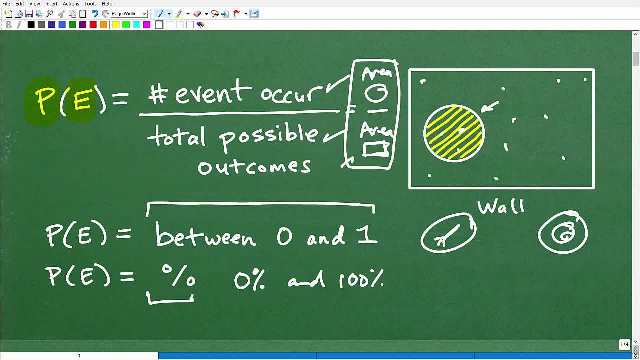 And so what we have here is some sort of fraction. okay, it's going to be something like, you know, one fifth, one third, whatever the case is, one seventh, 22 over 80, doesn't make a difference, It'll be some sort of fraction, okay, between zero and one, Okay. And then we want to go ahead and convert that fraction, which will be a decimal, all right, into a percentage. So it's just a basic review of probability here. And if we want to 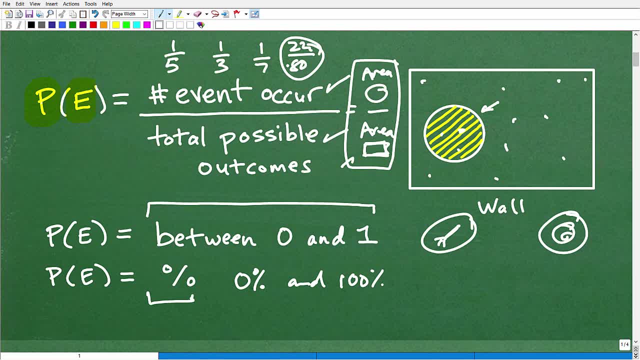 you're kind of lost. well, you know, maybe this problem won't make as much sense to you, but this is pretty, pretty basic stuff, so hopefully i explained it pretty well. uh, and again, i'm taking time to uh really emphasize probability, simple probability, with kind of figures like this, and 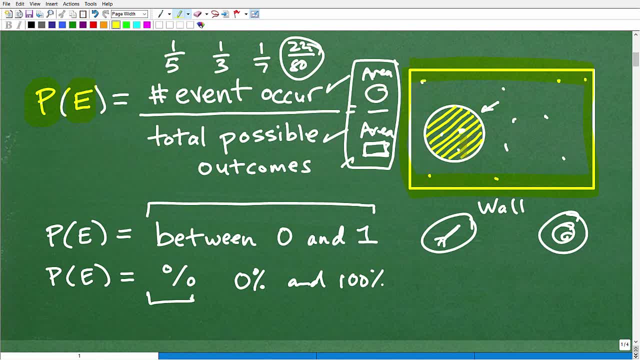 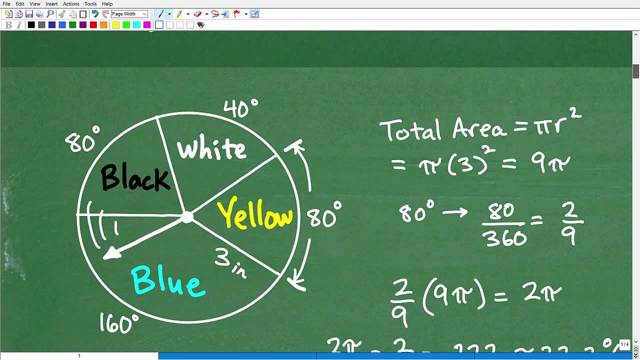 this is a common problem where there's like a rectangle or circle or like you know, different figures. okay, it's not just a normal kind of word problem, it's something graphically going on. this is how you handle it all, right. so, knowing that, let's get to our problem. okay, now one of the 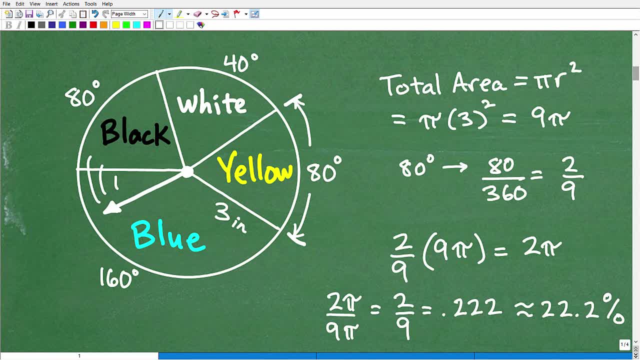 things that students do is they look at math. teachers love to do this. they give you a lot of information just to, kind of like, distract you, okay. in other words, they kind of put in excessive information, uh, and you don't need all that information, okay, to solve the problem. so here. 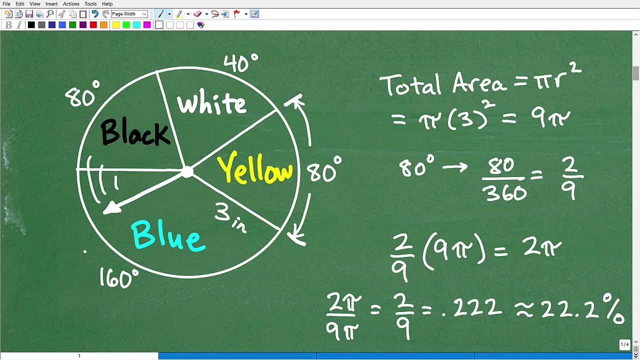 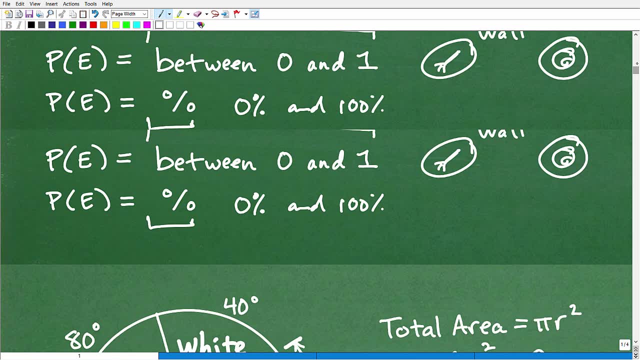 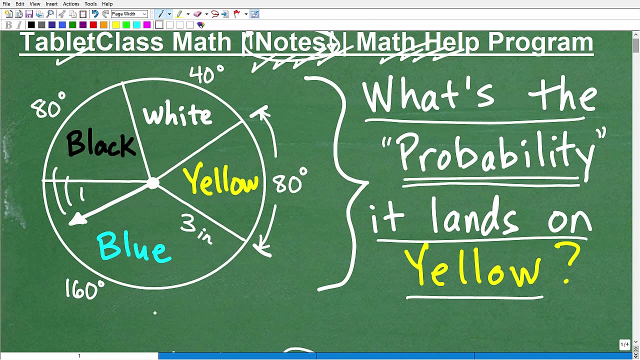 we have a lot of other additional information. i don't need to know about blue, black doesn't make a difference. i just need to know about yellow. so, from a graphical standpoint- okay, let me go up here, because i don't want to mess up that figure here- what we're really trying to do is determine is: i want to know the. 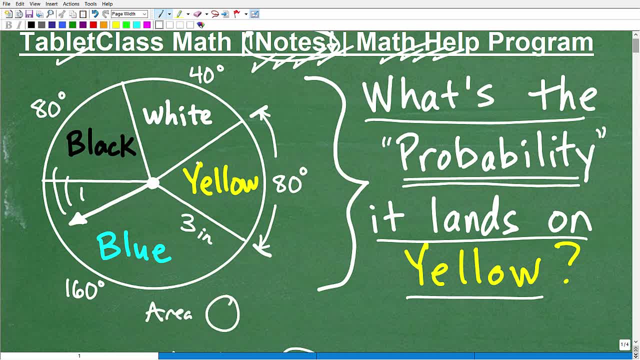 area of the circle, okay, and i would like to know the area of this right here, the area of the yellow sector, okay, so i want to determine these two things. so, the spinner, the probability that this will be the area of the yellow divided by the area of this of the total area of the circle, okay, 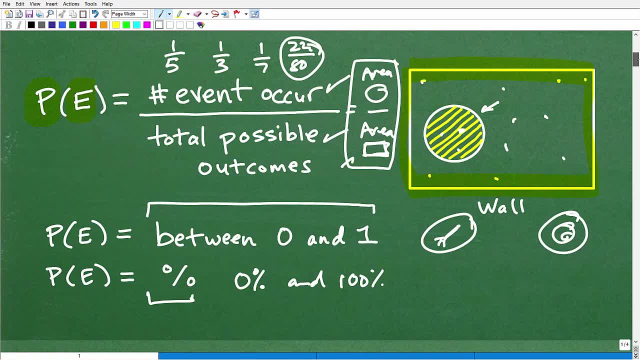 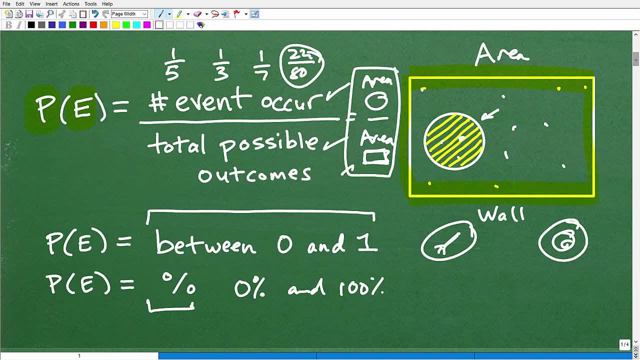 now there's another kind of more simplistic approach we can take to this, but i really want to emphasize this concept of using area, or finding area, to solve basic probability problems, especially things that are kind of graphically represented. okay, so here's our spinner, here's our. 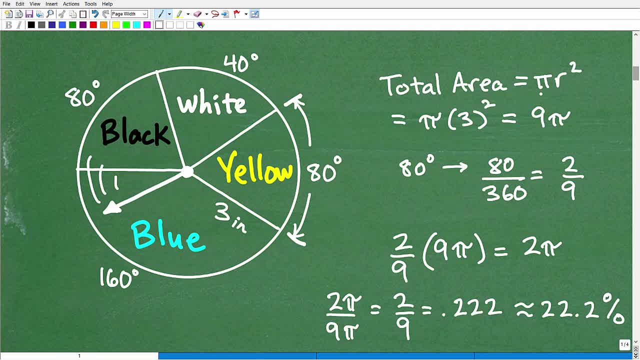 problem. so let's go ahead and figure out what the total area of the circle is. well, got to know how to find the area of a circle, and that's the area of the circle. and the area of the circle is the area of the circle, is our lovely formula pi r squared, it is the area, the formula for the area of a circle, so the area. 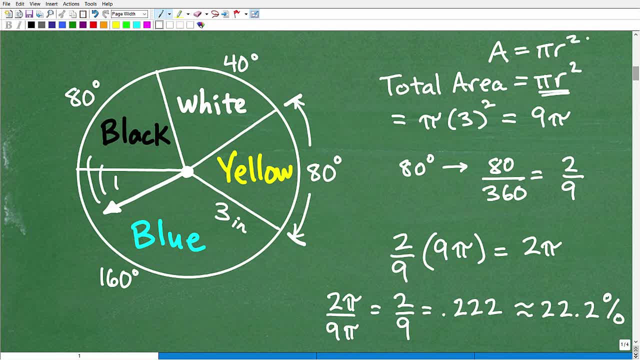 of a circle is pi r squared, something you should know or put into your long-term memory. so to find the area of this circle, i have to go look for more information. that would specifically be the radius. so here it is right. here there's three inches. so pi r squared, that's going to be pi the. 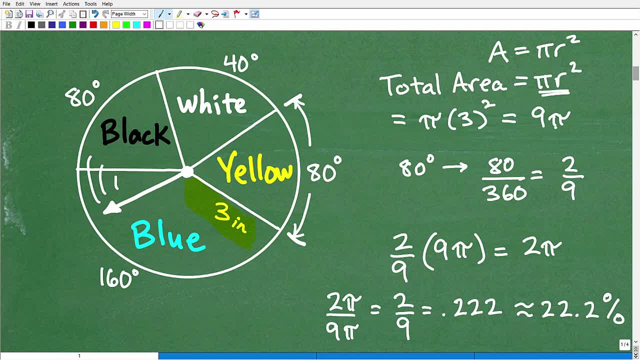 radius is three squared right. three squared is nine. so this would be nine pi inches squared, but we're talking about probability, so i'm just going to focus on that. nine pi, that's the total area of this circle. now, how do i find the area of this little arc here? i 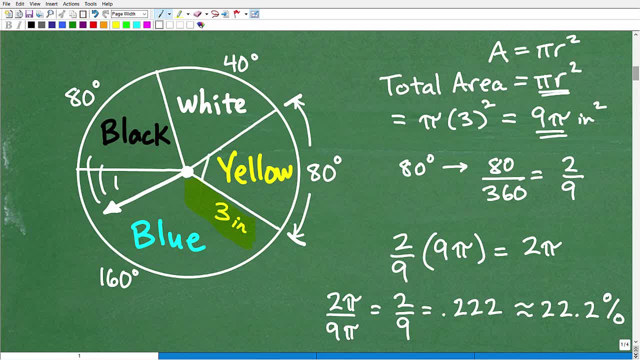 mean this little sector, little little piece of pi. okay, that represents the yellow portion, okay, of the circle. well, you can know a little bit about circles. now, how many degrees are in a circle? well, this isn't something else you should know. that's 360 degrees total. okay, so this is. 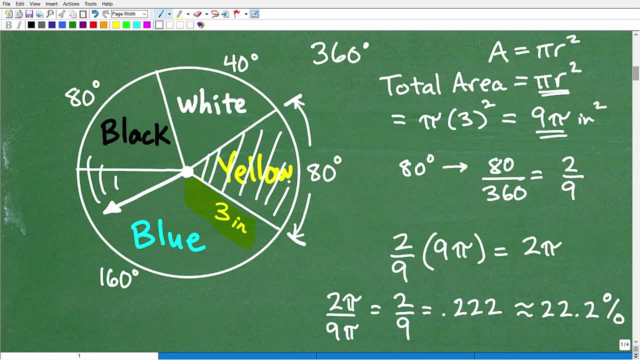 80 degrees. the circle is 360 degrees total. so this little sector here represents 80 out of 360 degrees of the circle. okay, which is the fraction two ninths. okay, so this area here will be two ninths of the total circle. so i could just take two ninths and multiply it by the area of the. 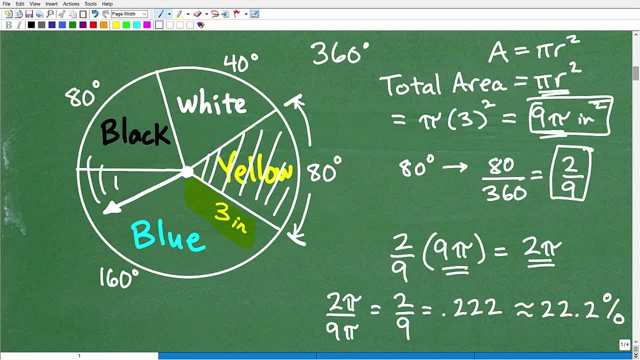 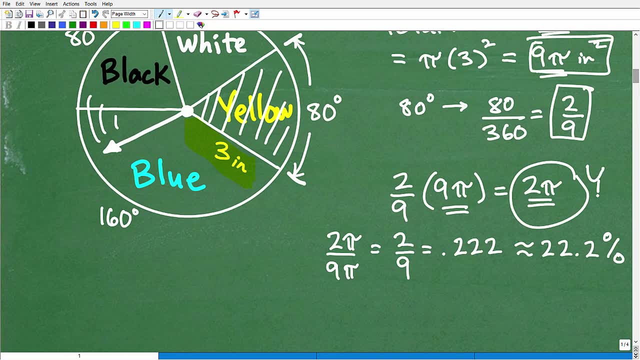 total circle and that is two pi. okay, all right. so now i know the area of the circle and i know the area. this is the area of the yellow sector. i know the total area of the circle, which is nine pi, so that's two pi. this is the yellow sector, over the total circle, the total right. so that's. 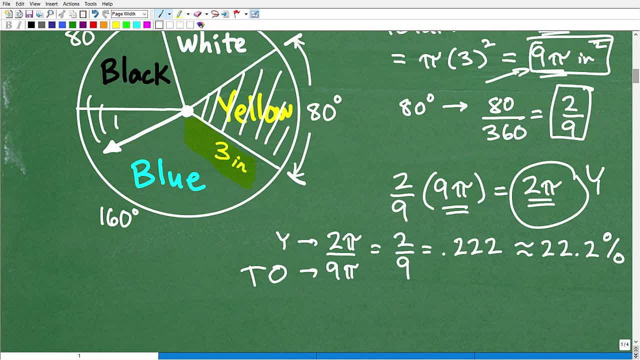 two pi over nine pi or two ninths? okay, when i take two divided by nine, you're going to get point two, two, two, two, repeating, okay. so again now here. this is our fraction, this is the definition of probability. this is a number between zero and one, but, as i told you, we like to represent a percent as a decimal. so we're going. 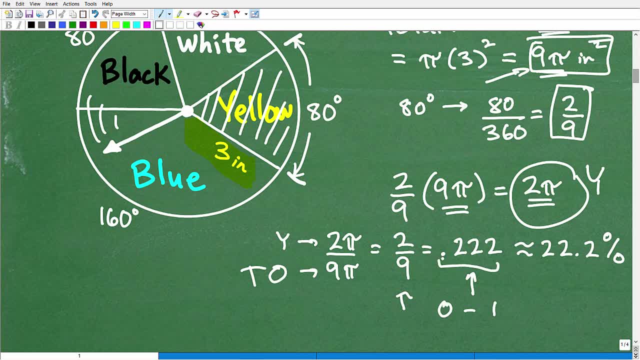 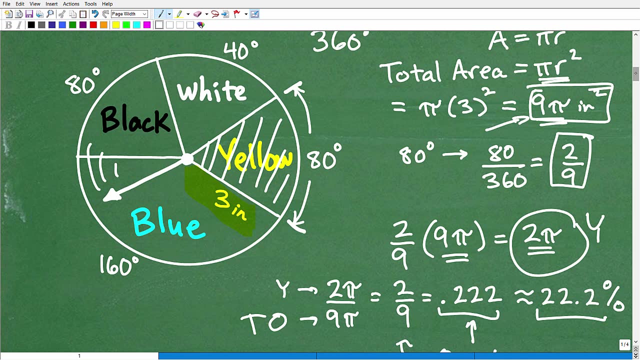 to take our answer and multiply by 100 or scoot the decimal point over two places to the right, it's the same thing and that is 22.2 percent. okay, so that is the probability. the probability that the spinner will land here would be 22.2 percent. now somebody out there could say like: 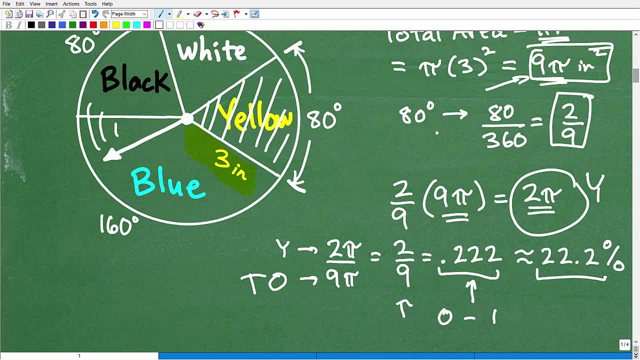 well, i don't need to find the area of the circle, i could just know that, um, right here. uh, this represents 80 out of 360, and that would be two ninths. and then i could go ahead and convert that to a decimal, and that would be fine too. okay for this particular problem. 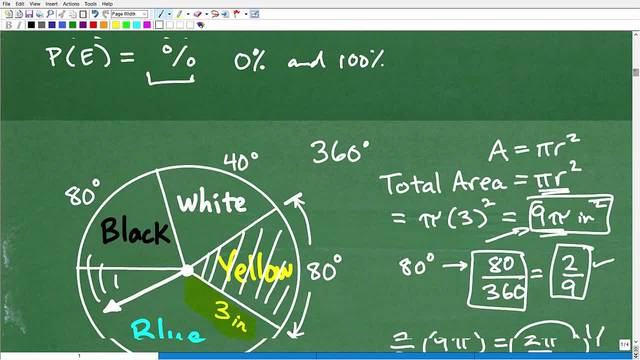 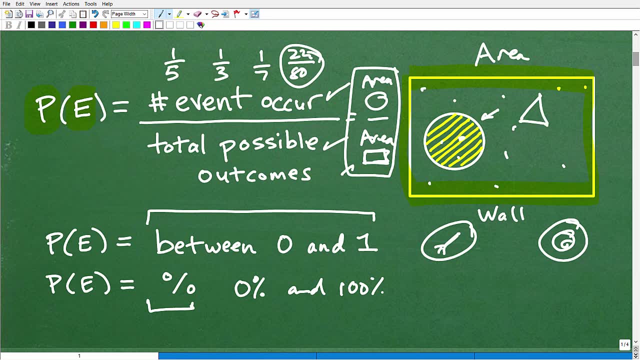 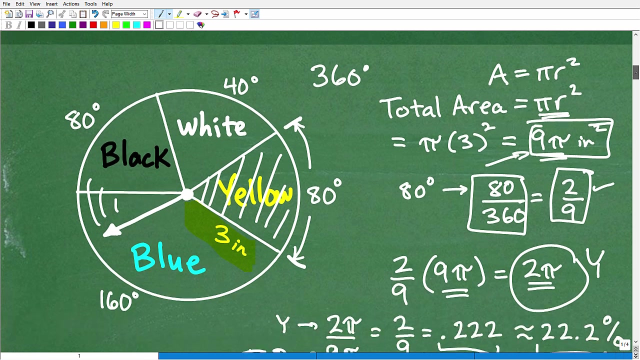 that would be okay too, but i wanted to um stress that, in problems like this, where you have a circle and a rectangle or a triangle- okay, things like this- is a very common type of- uh, uh, probability problems, simple probability problems. you have figures, you have no alternative other than to calculate the area. okay, all right now. one other thing i wanted to mention. 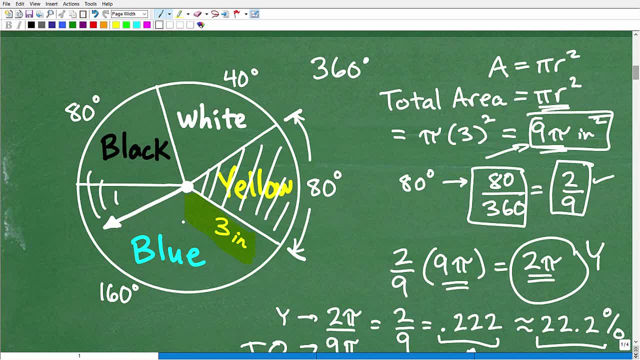 on here as well, is that. you know some students might be like: okay, i got the yellow, maybe i need to find the? uh, find the area of all these other little things, those little sectors. here too, remember a lot of math problems. they'll give you a lot of extra information. you got to be very 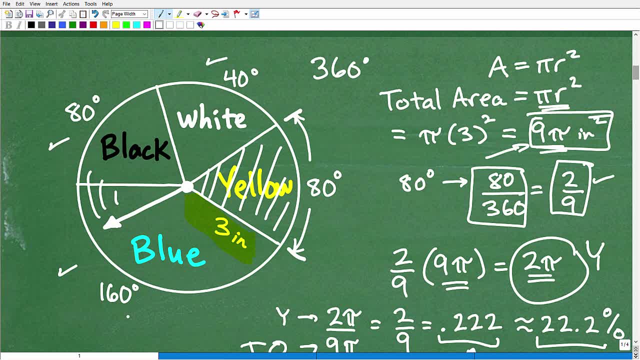 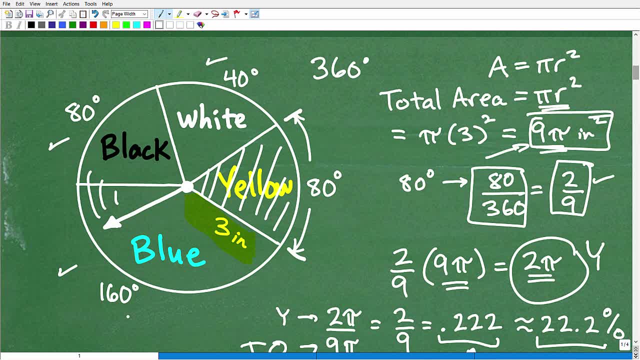 do, or math test, especially standardized tests. they'll give you additional information. it has nothing to do, just extra stuff, and they're really just trying to confuse you, okay. so always read the prompt carefully and focus in on what you need, and only focus in on what you need.